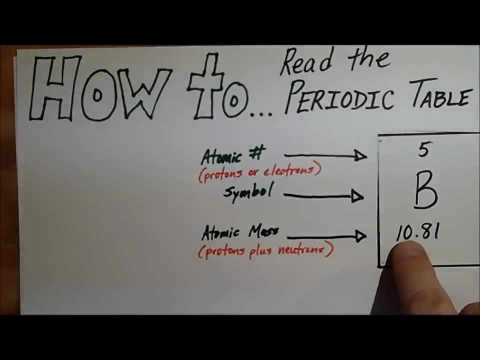 this to a whole number, In this case up to 11.. And then what you're going to do is subtract out the protons, So you take 11 minus 5. And by doing that it gives you 6., And so that tells you the number of neutrons. 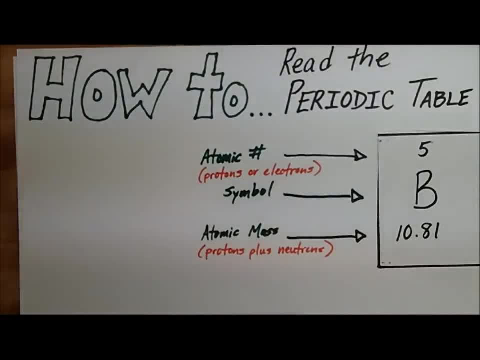 You have 6 neutrons for this atom. If we take a look at the atom, here's a picture of the shells And we'll look at the electron configuration, or what's called the Bohr diagram. And for this one let's take a look at the. Let's think about the nucleus In a nucleus. 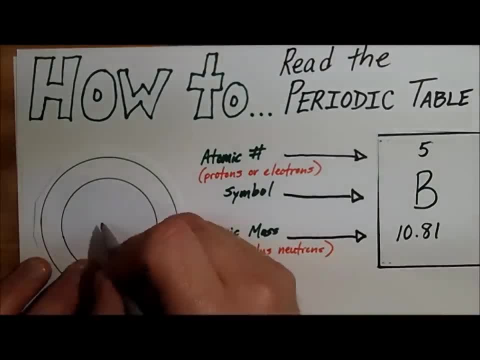 that's where you're going to have the 6 neutrons and 5 protons. So in that nucleus I'm going to have 5 protons- I'll put a plus here because they're positive- And then 6 neutrons. I'll 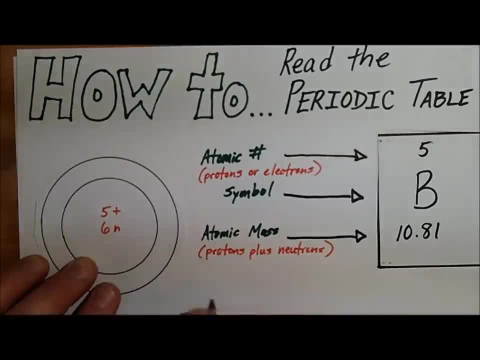 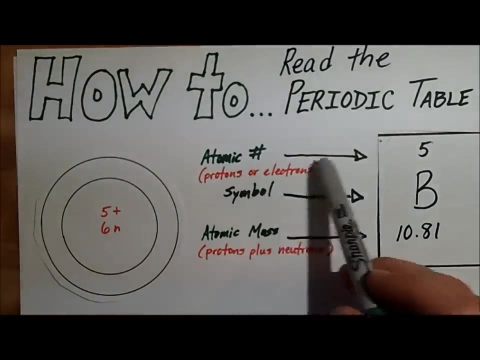 put an N for that. So that's in the center, in the nucleus Surrounding that, you have a cloud of electrons spinning really fast, So fast that you can't really even see them. They'd be a blur, And so those electrons will be the same number as the protons, So we're 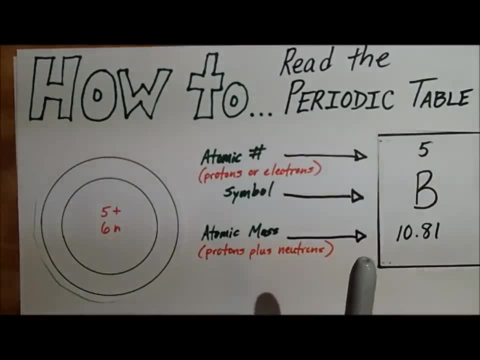 going to have 5 of those spinning around, And as they spin, They're going to be in these different shells. Now there's some rules that you need to know about the shells, And the rules for the shells are the following: This is a basic set of 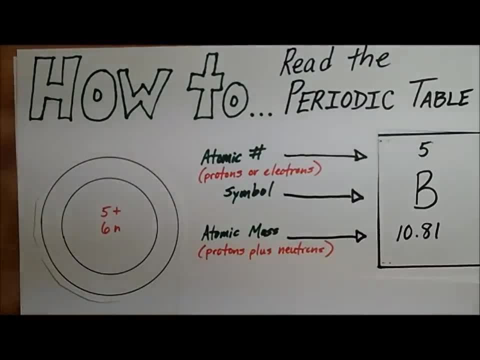 rules that can help you figure out the Bohr diagram. So this first shell, starting on the inside, working our way out, I'll put the little chart here: Shell number. Shell number 1.. Shell number 2. Shell number 3. Shell number 4. Shell number 5. Shell number. 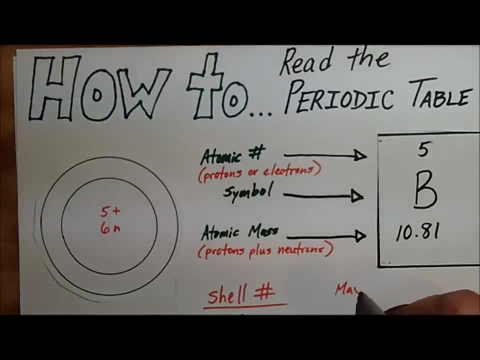 1. Shell number. 6. Shell number, 7. Shell number 8. Shell number, 9. Shell number, 10. Shell number 8.. And the maximum electrons. That's the symbol for electrons, Maximum electrons it holds. So the first shell can only hold 2 electrons, 2 electrons. The second shell, 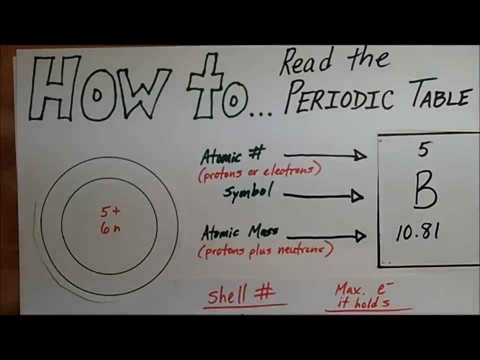 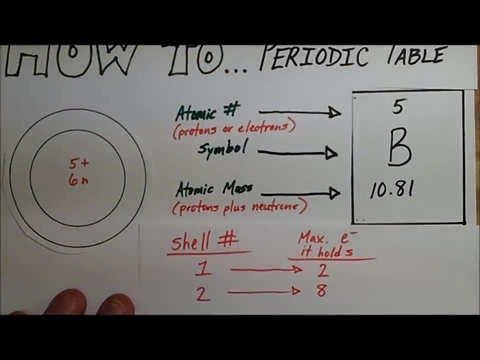 will hold up to 8.. Let me move this up so you can see it a little bit. Here we go, Okay, So first shell holds 2.. Second shell holds 8.. Now, when you go to the third shell, it starts to get a little tricky, because there's something. 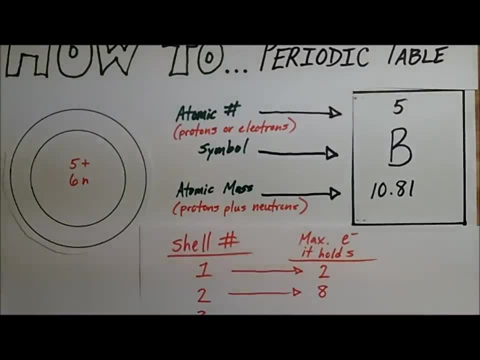 called sub-ordinals that are involved, But what you're going to do is just remember the number 8.. Because the elements want to feel like they have 8 on their outer shell, on the third shell shell. They do add other shells as they get larger and it gets a little more complicated. 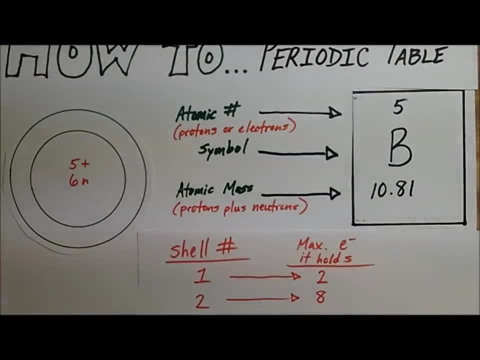 than that, but in a simplified version. what you need to remember when filling out these bore diagrams is, especially with the first 18 elements, is: remember 2, 8, 8.. This one actually holds 18, but you want to remember this number 8.. 8 is kind of the magic number. 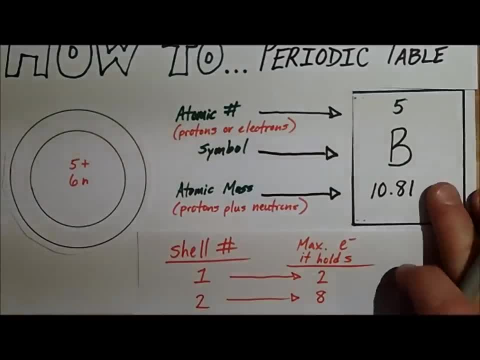 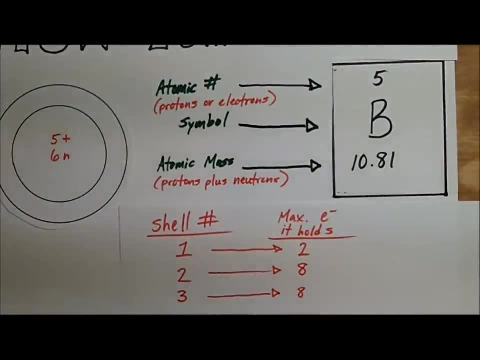 It's something called the octet rule where the elements prefer to have this 8 on the outer shell of the third shell and the fourth shell and the fifth shell and the sixth shell. But I'm not going to get into the sub-orbitals and that electron configuration with this. 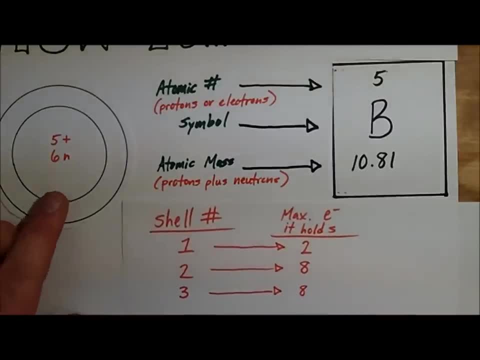 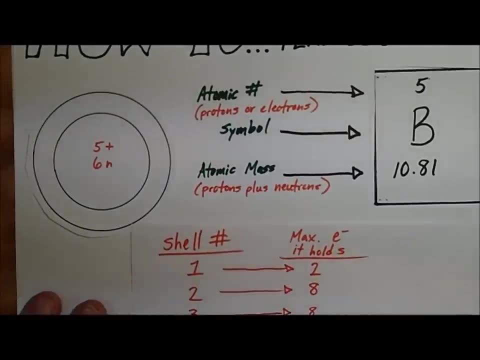 Okay. so, moving on from that, let's take a look at how do you put the electrons. how do you put these electrons following these rules? how do I put the electrons where they need to go? Okay, So I'm going to take this away for a second. 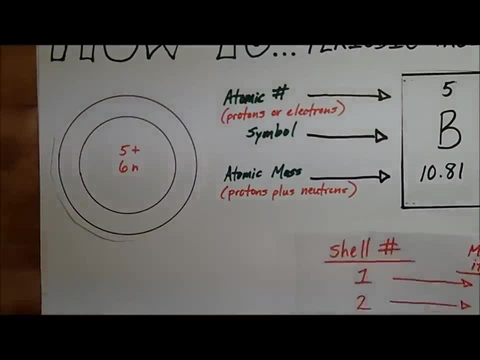 First, we've got to remember that the electron number will be the same as electron number is going to be the same as proton number. So we have 5 electrons. I'm going to do them in a different color here, I'll just use green. So we have 5 electrons spinning around Only. 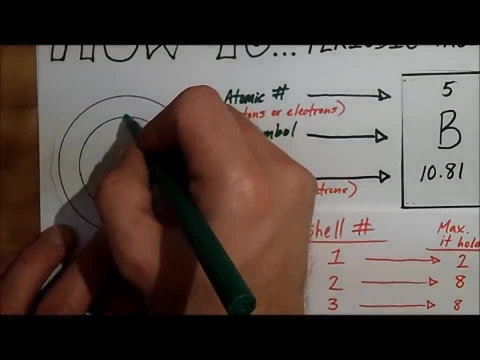 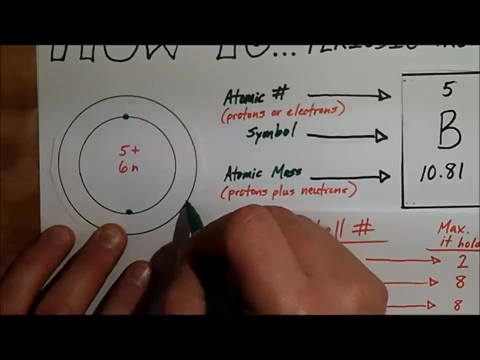 2 can fit in this first shell, So I'm going to put them here for a shell. There's 2.. The rest, let's see. I have 3 more because I have 5 total. The rest are going to go on. 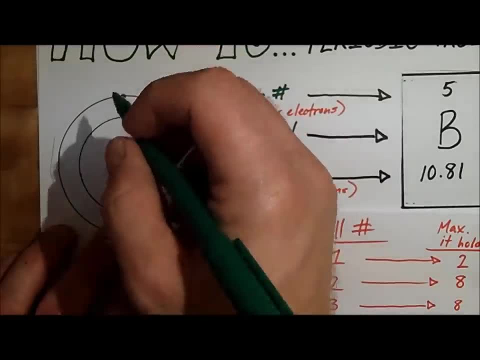 the second shell. The shell- another name for the shell- is the second shell, So I'm going to put them on the second shell. The second shell is also called an orbital or energy level- A couple of different names, So it doesn't matter where you put them on. 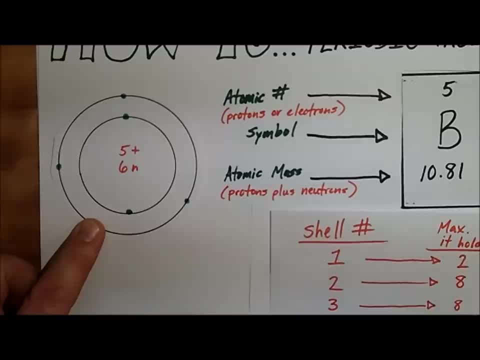 the shell on the circles because in reality they're actually spinning really quickly. So I have a total, as you can see, of 1,, 2,, 3,, 4,, 5.. And now I'm done with that electron.